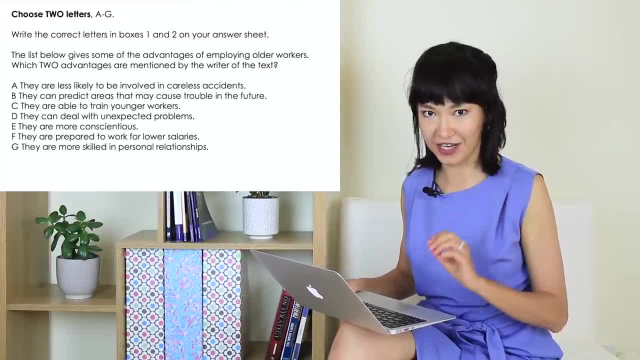 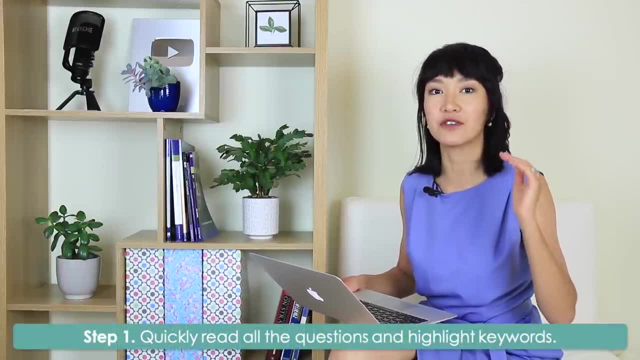 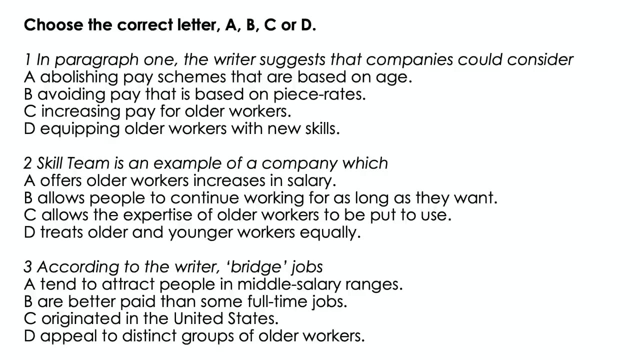 options and you need to choose two correct options. When you see these questions, the first step is to quickly read all multiple choice questions and highlight keywords. Let's have a look at our three questions. In paragraph one, the writer suggests that companies could consider: 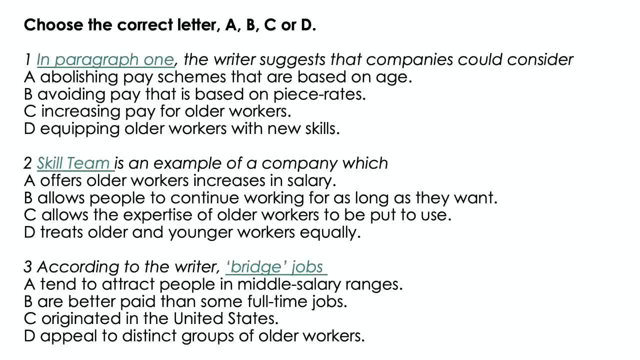 So the keywords are in paragraph one. They will help us to locate the answer. Question two: Skill team is an example of a company which The keywords are: skill team. Question three: According to the writer, bridge jobs, The keywords are: 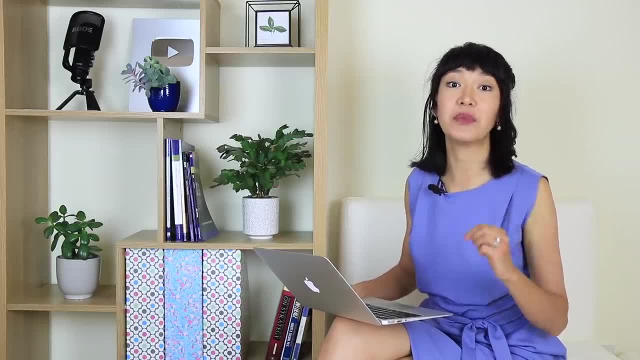 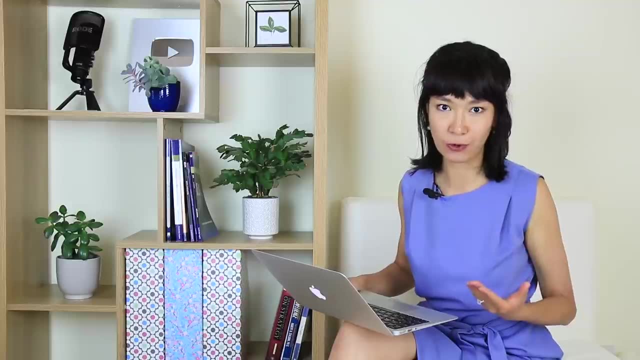 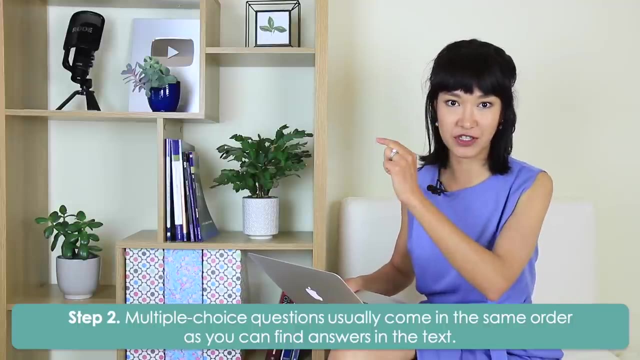 Bridge jobs. So the keywords will help me to locate the answers. That's all I need for now. The second step is just something you need to know. Multiple choice questions typically come in order. It means you can read the first question. start reading the passage until you find the answer. 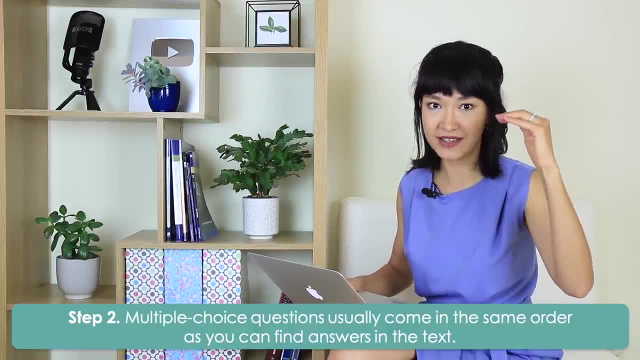 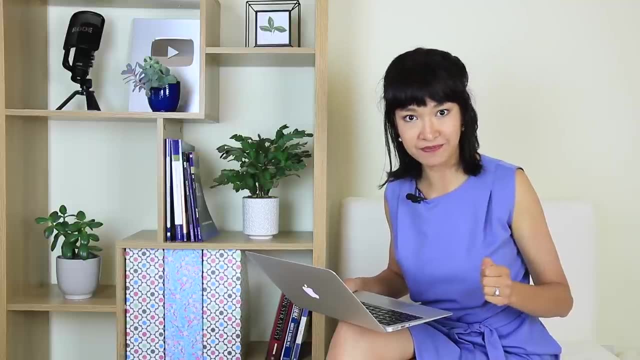 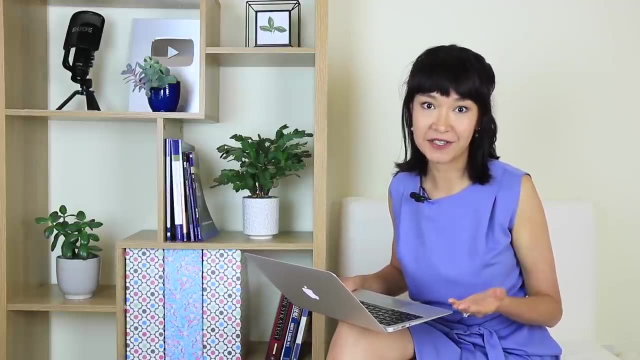 Then you read the next question, you resume reading the text until you find an answer, and so on. Many questions include in IELTS reading actually come in order, But some don't, And if you know which do and which don't, it's a huge time-saver. I have a separate video about them and 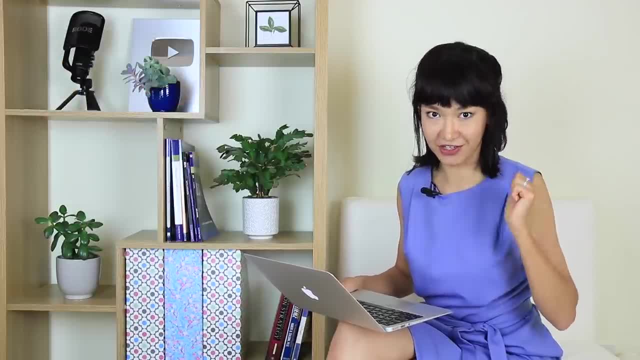 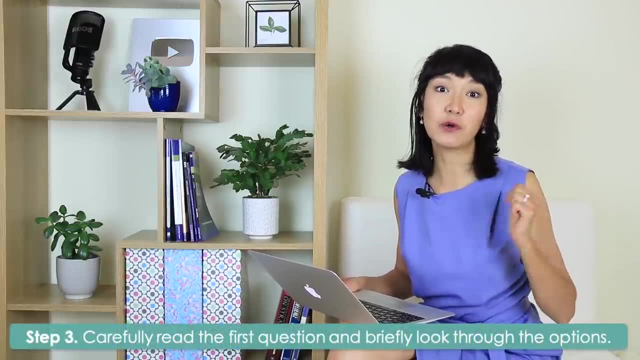 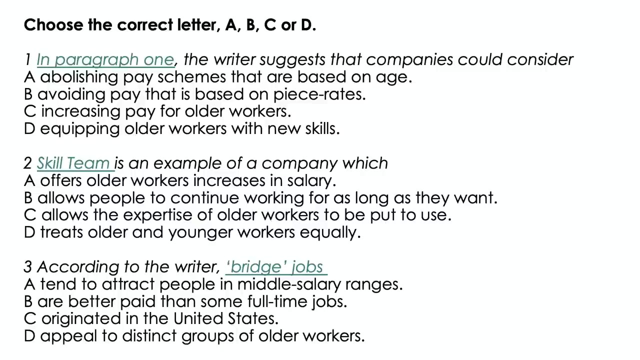 all the videos I mentioned are gonna be linked in the description. Step number three: Carefully read the first question and quickly look through the options. Our question is In paragraph one. the writer suggests that companies could consider. So we know the answer is in the first paragraph And I've copied. 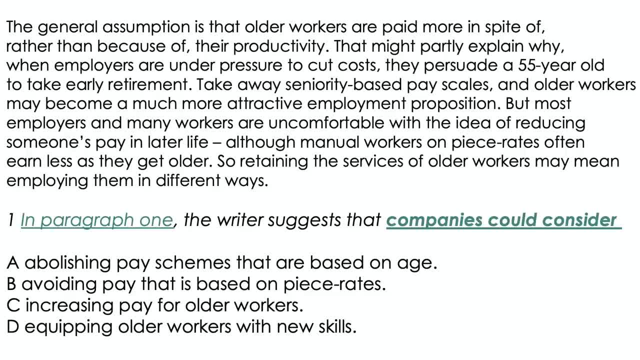 the first paragraph and the question onto this new slide. So we are looking for what the companies could consider And I will just quickly look through the options. I don't need to memorize them Just to get an idea of whatever the options are. I don't need to memorize them just to get an idea of. 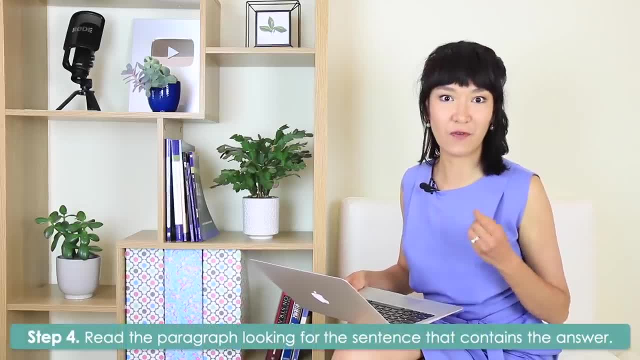 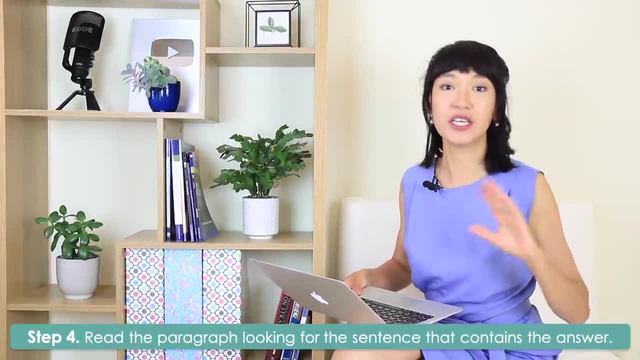 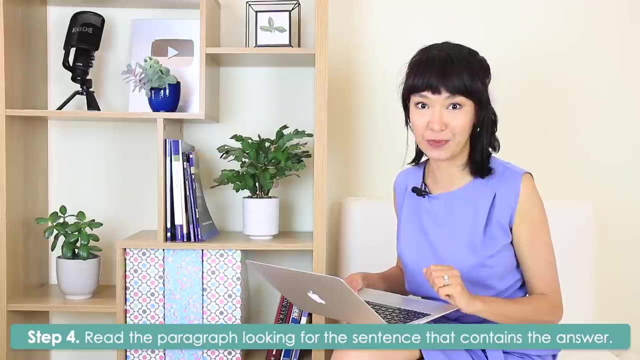 what I can find here. Step number four: Read the passage trying to find the answer. If you don't know what the answer is, don't worry, Just try to find this bit in the paragraph, maybe this sentence, where the answer is likely to be Now I 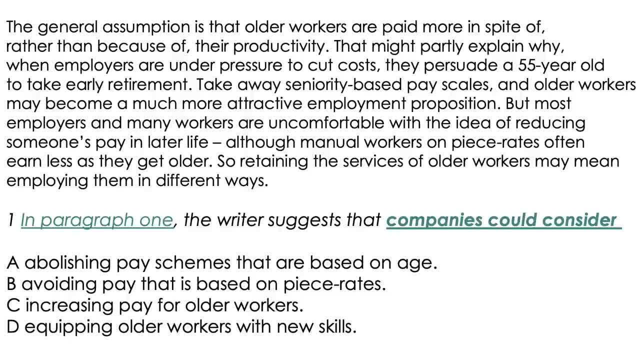 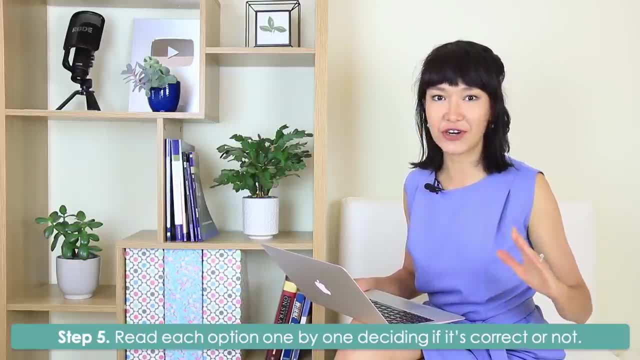 want you to pause the video, read the paragraph and try to find the answer, and then resume the video Done. Step number five: Read each option one by one, deciding if it's correct or not, And I have a few tips. First of all, highlight. 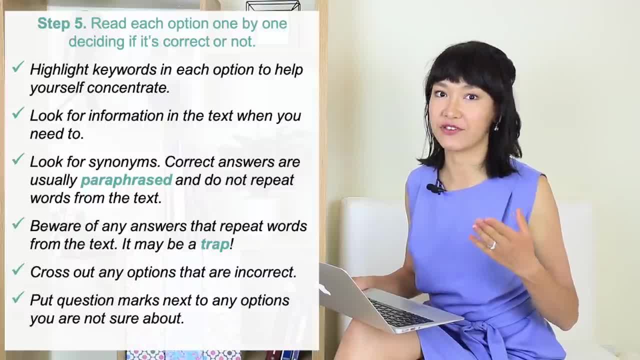 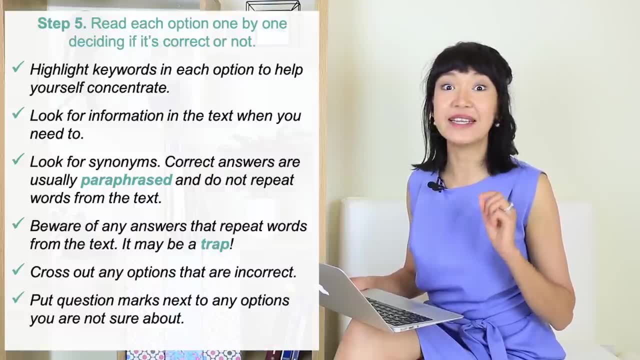 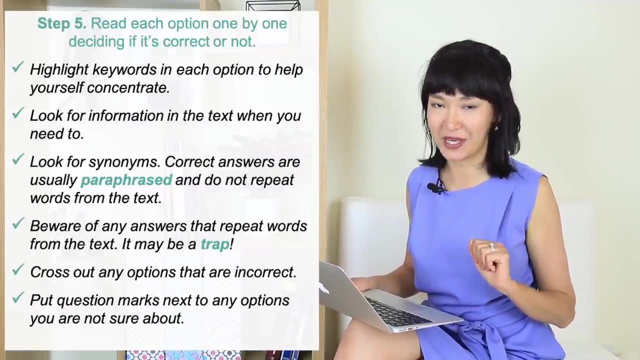 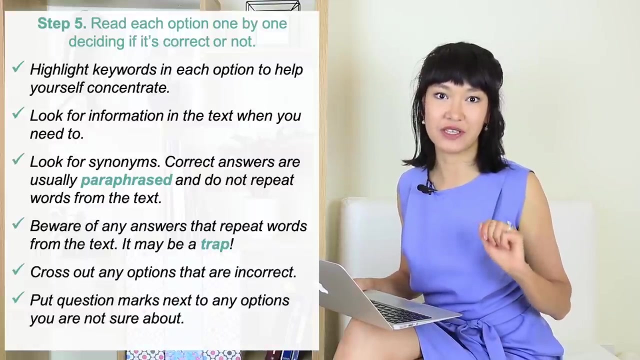 keywords in each option to help you decide if it's correct or not. Look for information in the paragraph when you need. Look for synonyms as words in the text and in the option. Topics are usually paraphrased and are not repeated. particularly incorrect answers. Cross out any options that are incorrect, straightaway and put. 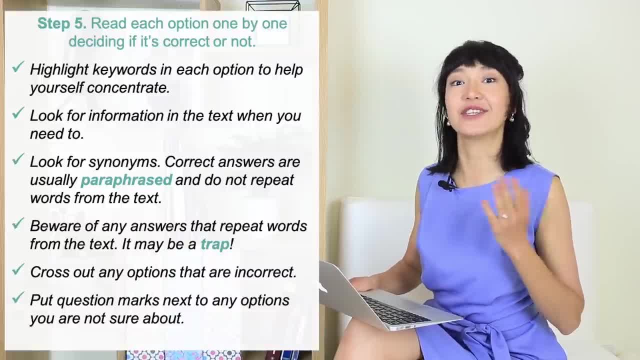 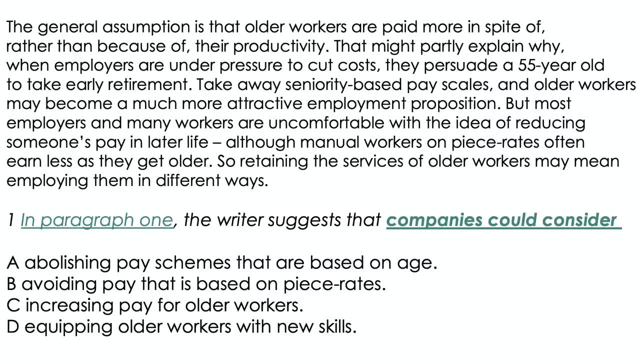 question marks next to options, which may be correct. if you are unsure and want to come back later, Let's look at our options. Option A: Abolishing pay schemes that are based on age. So we are looking at an example of the fact that the answer to this question is correct or wrong. 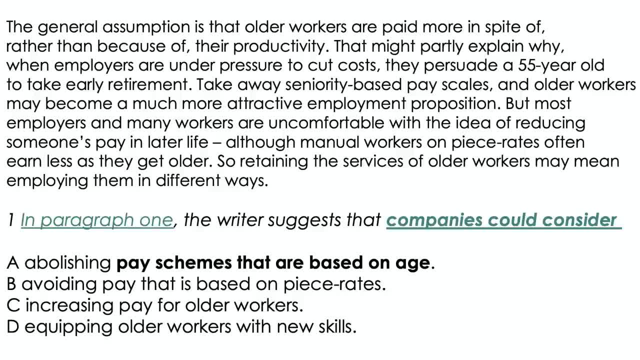 Now let's go back to the previous question. Let's look at the previous question. Let's look at the previous question. What is the answer to this question? looking for synonyms in the text and I found seniority based pay scales. Let's 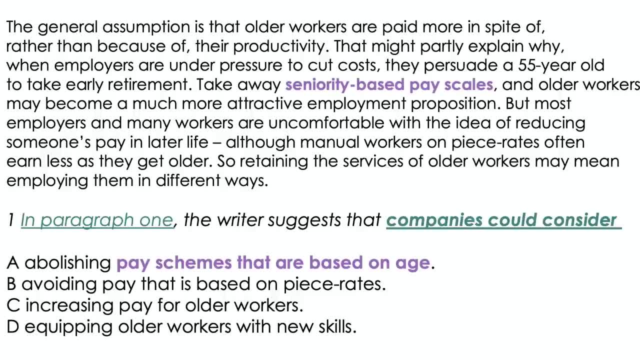 compare them. Seniority is related to age right, And abolishing is the same as taking away. So what do we get? Companies could consider taking away seniority based pay scales or abolishing pay schemes that are based on age and older. 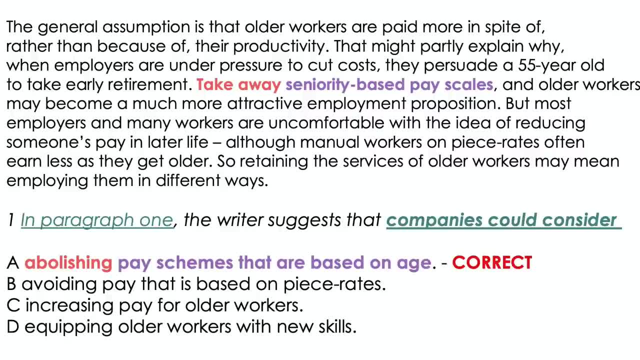 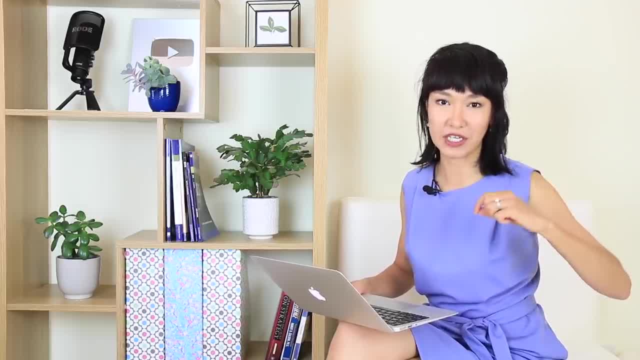 workers will become more attractive, So they could consider that right. That's the correct answer. As soon as I get the answer, I mark it and move on to the next question. But if you're still unsure, you can check each option and cross them out. 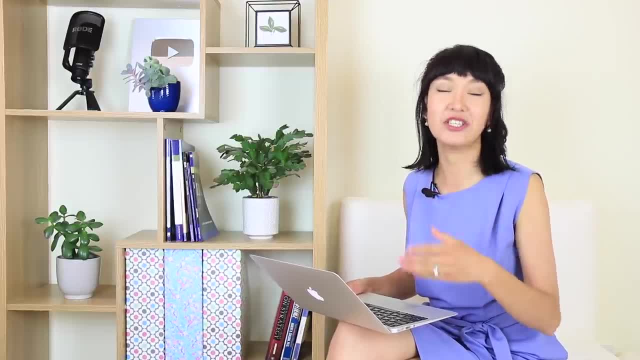 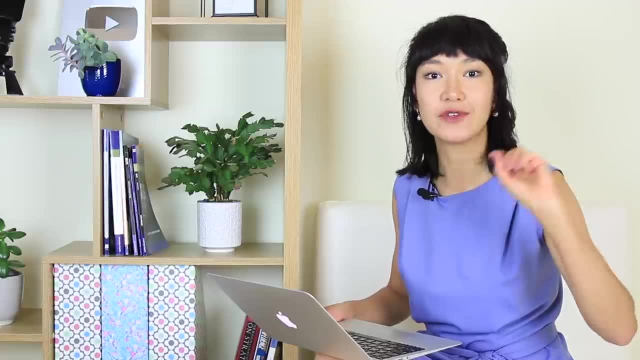 until you'll be left with option A, but it just takes more time. so only do that. if you aren't sure, In a paper-based exam you can cross out options on the question sheets, but if you take a computer-based exam, you can. 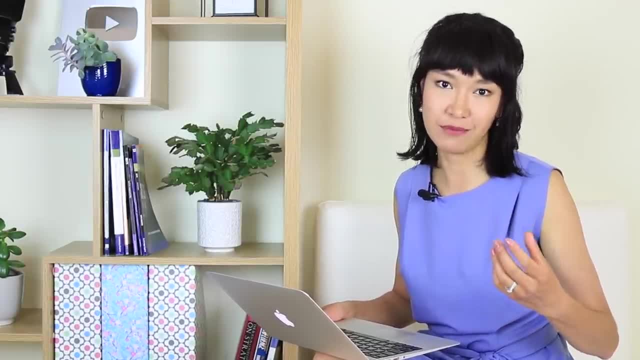 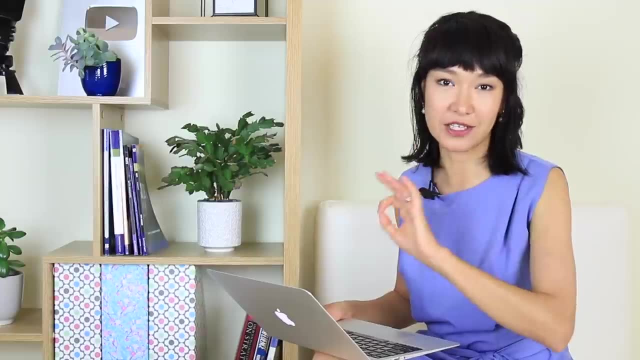 use a highlighter, but then it takes a bit of time. You need to click a couple of times to highlight something. You can also use pen and paper to mark answers which are incorrect or answers which you think might be correct. Let's move on to. 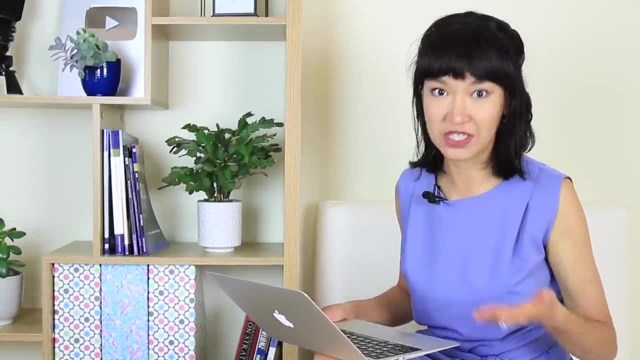 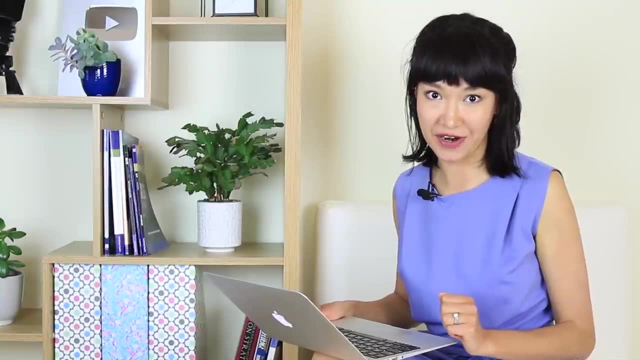 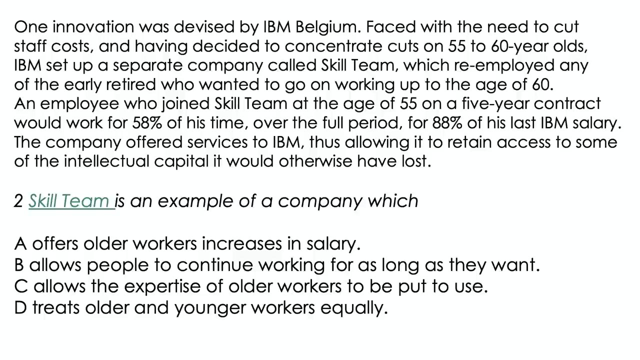 the next question. We know that questions come in order, step two. so the answer to the second question most likely will be in the second paragraph. Let's have a look. I've copied the second paragraph and the second question on the same slide. Let's go back to step number three. 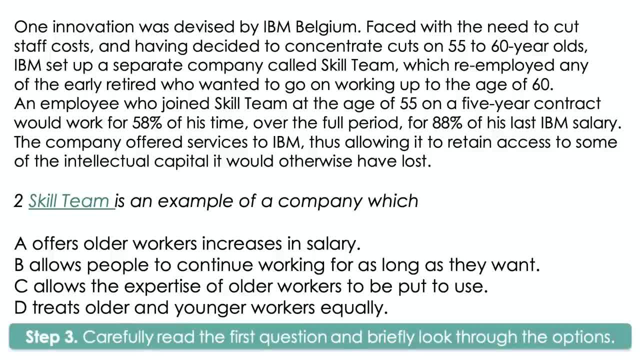 Carefully read the question and look through the options. briefly, Our question is: skill team is an example of a company which? So we are looking for the definition of a skill team. Step number four: read the text looking for the answer. Please pause the video, read the text and try to find. 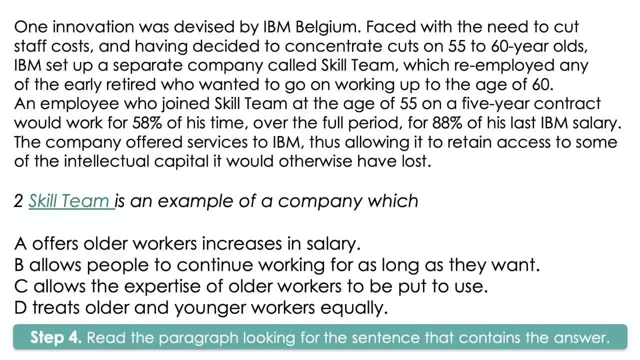 your answer and then resume the video. Could you locate the answer? After reading the paragraph, I've realized that the whole paragraph is about the skill team, so it's definitely the correct paragraph, but we can't really say where exactly the answer is. Step number five: Let's read each option and decide if it's correct or not. 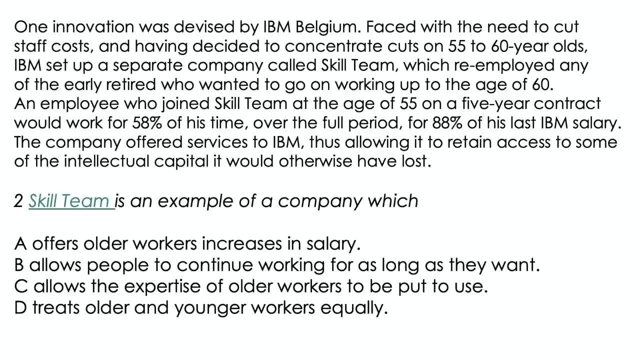 Option A offers older workers increases in salary. The key words are increases in salary. Is it correct? Let's look for the answer in the paragraph. I can find this bit For 88% of his last IBM salary. So the salary will be lower, not higher. There is no increase, So it's incorrect. Cross it out. 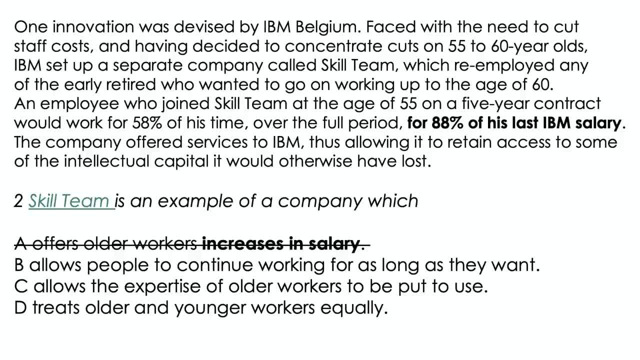 Option B allows people to continue working for as long as they want. The key words are to continue working as long as they want And in the paragraph I can find, to go on working up to the age of 60. So that's not as long as they want. Again, this option is incorrect. Cross it out. 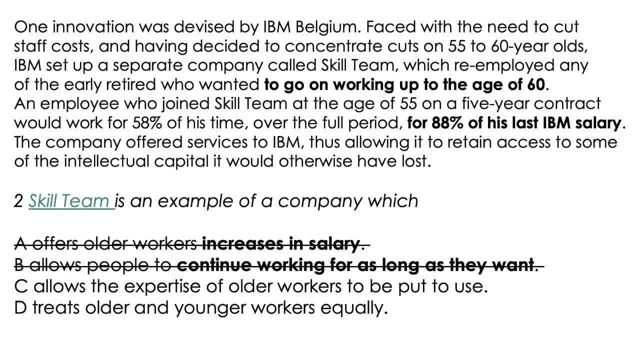 Option C allows the expertise of older workers to be put to use And in the paragraph I can read: allowing it to retain access to some of the intellectual capital, And intellectual capital is their expertise right, And to retain access is the same as to be put in use. 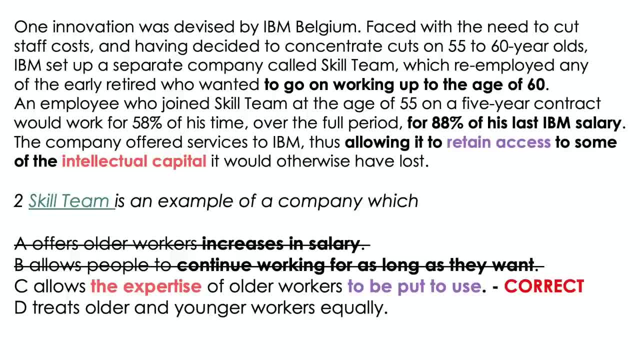 So that's the correct answer. What about D? Treats older and younger workers equally? I don't remember reading anything about younger workers at all And I'm not gonna look for it, because I'm quite certain that C is the correct answer. 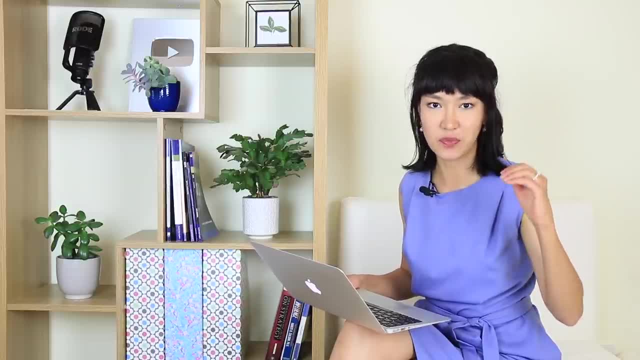 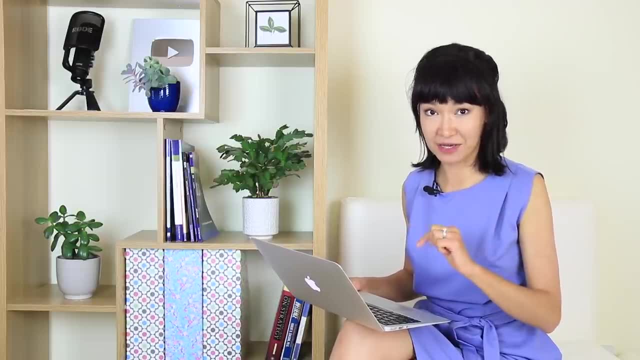 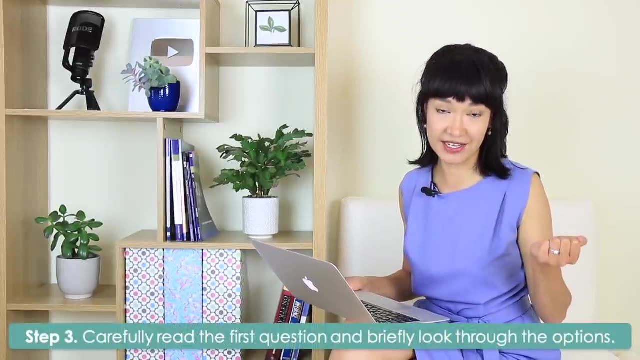 Next The second paragraph, and the whole paragraph was about skill team, So it's likely that the next answer will be in the next paragraph. I'm gonna copy it to the same slide and let's go back to step three. Carefully read the question and quickly look through the options. 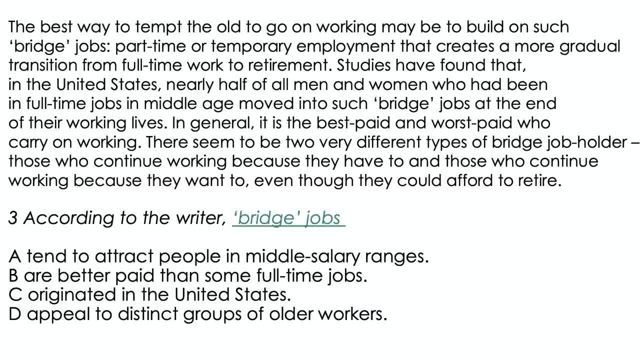 Our question is, according to the writer, bridge jobs, And we have several statements about bridge jobs And we need to find one that is correct. Step number four: Read the paragraph looking for the answer and don't worry if you can't see it straight away. 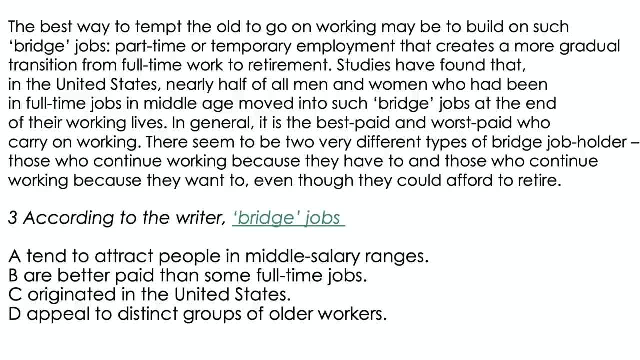 Please pause the video, try to find the answer and then resume it. Let's look for the answer together. Step five: Read each option, deciding if it's correct or not. A- Tend to attract people. B- Work in middle salary ranges. 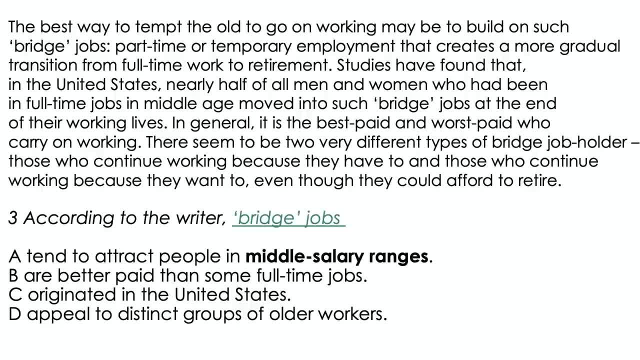 The keywords are middle salary ranges And we'll look for the information in the paragraph I can read: It is the best paid and worst paid who carry on working. So A is incorrect. Cross it out. B Are better paid than some full-time jobs. 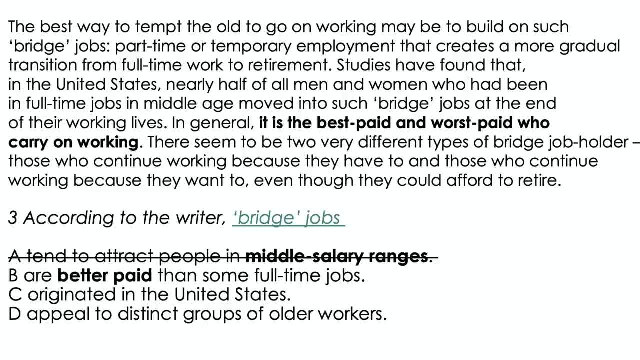 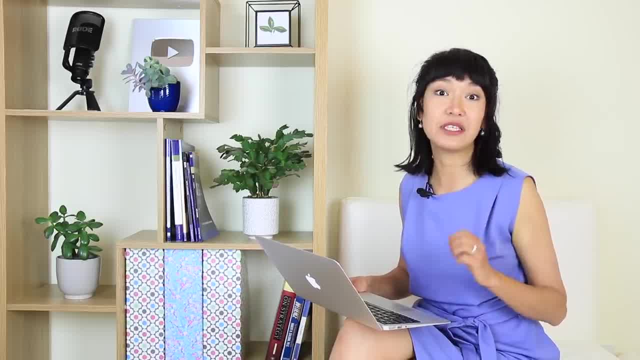 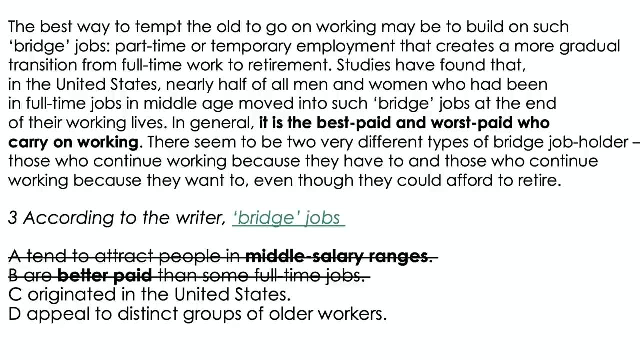 The keywords are better paid. I can't find anything about it. Sometimes the information is contradictory, But sometimes it's simply missing. In any case, it's incorrect. Cross it out: C Originated in the United States And the keyword is originated. 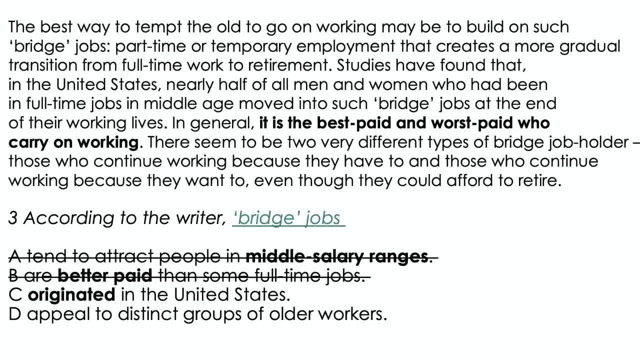 It means bridge jobs first appeared or were invented in the USA. I can find in the USA nearly half of all men and women who had been in full-time jobs in middle age moved into such bridge jobs. But we don't know where bridge jobs originated. 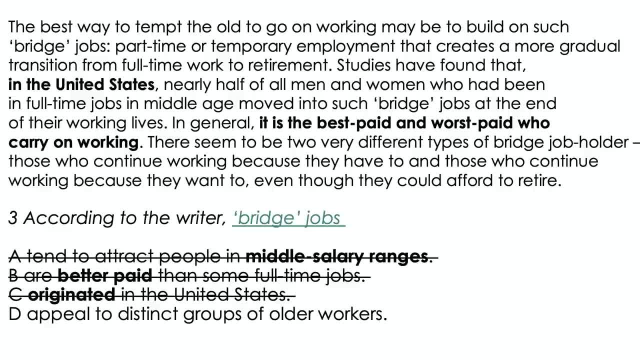 Again, the information is missing and this option is incorrect, So D must be correct. C: Appeal to distinct groups of older workers. And in the paragraph I can read: there seem to be two very different types of bridge job holder And if we compare them, distinct means very different. 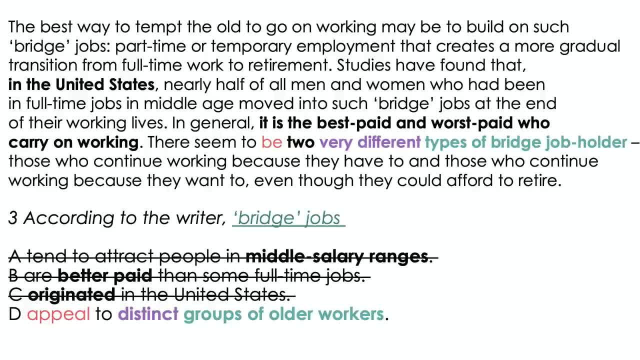 Groups of older workers are types of bridge. job holder Appeal is the same as there seems to be. So you see, the idea is absolutely the same, But words are different. Words are not repeated, So this is the correct answer. 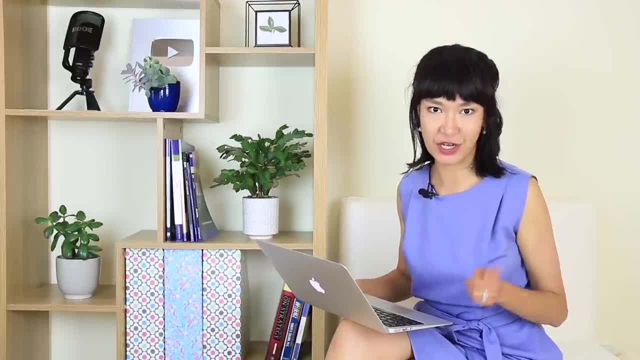 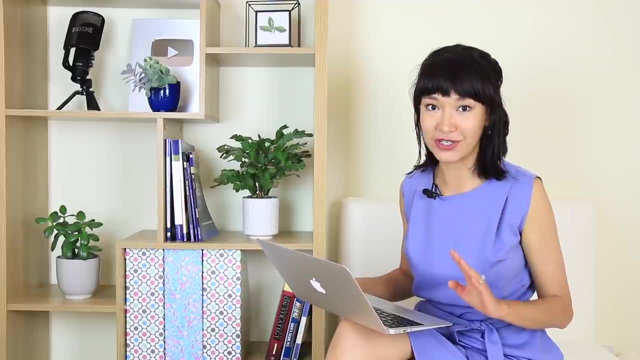 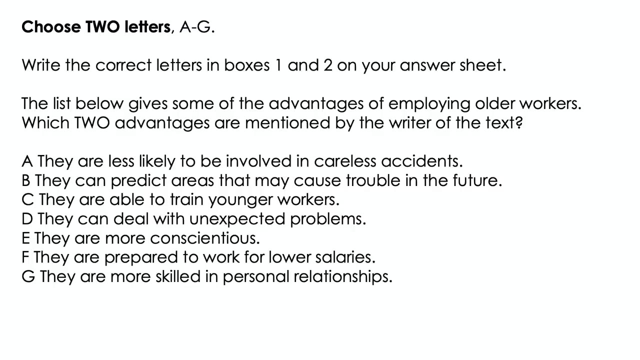 These were questions with four options And one correct answer. There is a slightly different type of multiple-choice questions with seven options and two correct answers. Let's have a look at one. First of all, carefully read the task Here. it says: choose two letters. 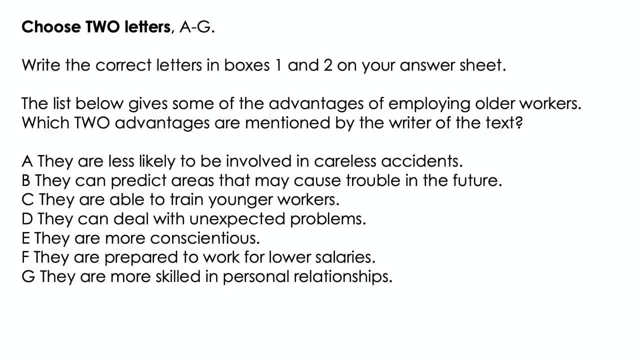 And we use our five-step plan, Step number one: Quickly read the question and highlight keywords. The question is: The list below gives some of the advantages of employing older workers. Which two advantages are mentioned by the writer of the text? The keywords here are two advantages. 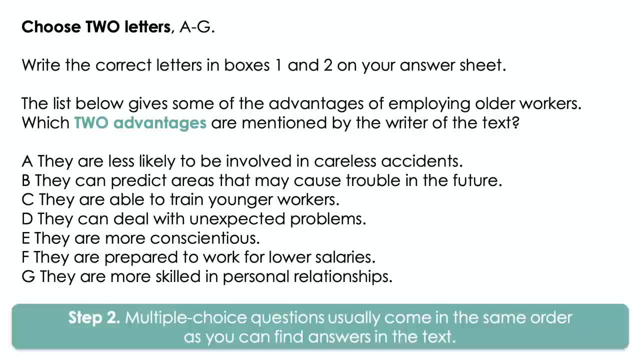 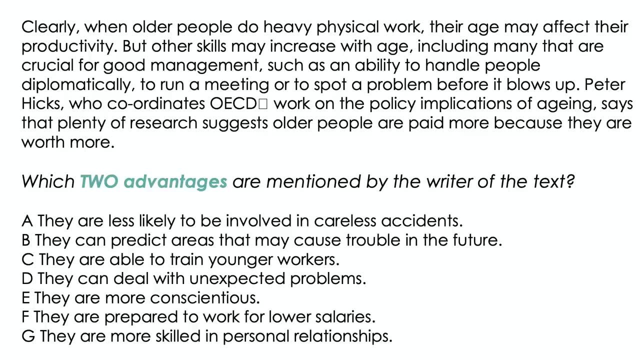 That's what we're looking for. Step two: We know that multiple-choice questions usually come in order, So it's likely that the answer is going to be in the paragraph we haven't read yet, So I've copied the next paragraph and the question on the same slide. 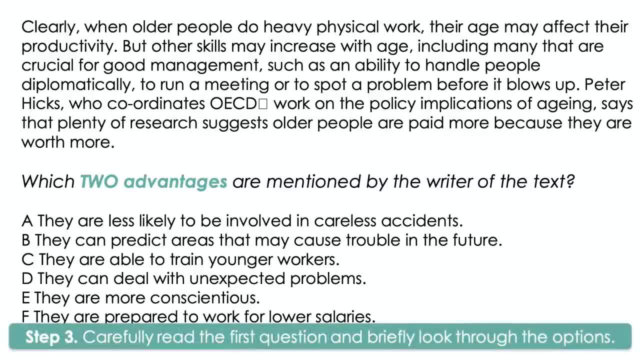 Step three: Carefully read the question and look through the options. briefly, Again, we are looking for two advantages And we just scan through the options without reading them too carefully for a few seconds. Step number four: Read the paragraph looking for the answer to the question. 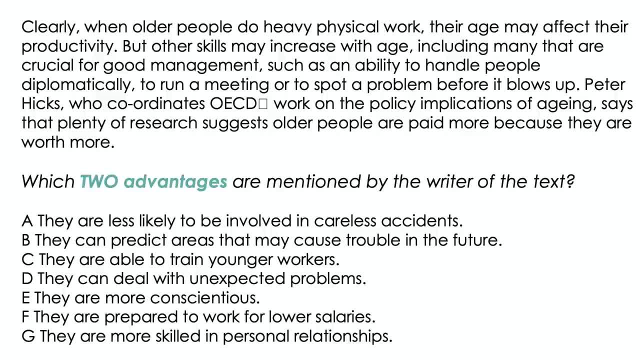 Please pause the video and try to find the answer Ready. I haven't found the exact answer, but I've found this sentence where the answer should be: But other skills may increase with age, including many that are crucial for good management, such as an ability to handle people diplomatically, to run a meeting or to spot a problem before it blows up. 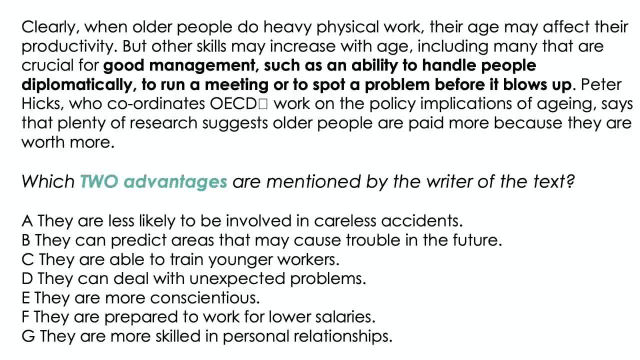 Highlight this relevant bit of the text. Use a pencil in a paper-based exam and a yellow highlighter in a computer-based exam. Step number five: Read each option, deciding if it's correct or not. They are less likely to be involved in careless accidents. 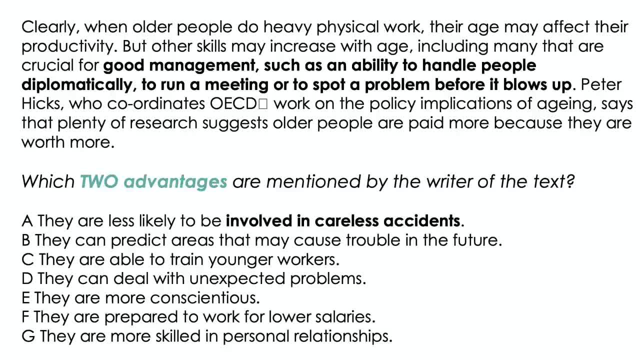 Keywords are involved in careless accidents. Compare it to the paragraph, especially to the bit. we've highlighted Nothing, So it's incorrect option. They can predict areas that may cause trouble in the future. Got it. Trouble is similar to problem in the text. 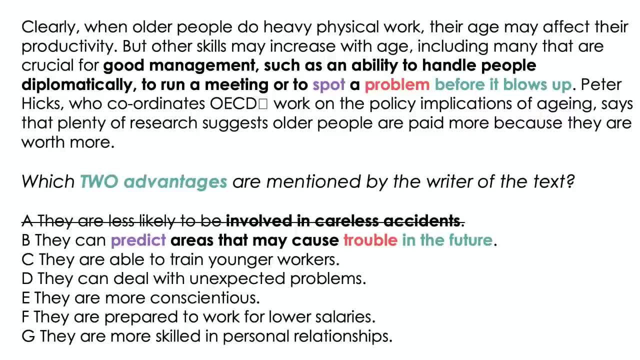 And if we compare the rest, predict trouble is to spot a problem In the future is before it blows up. So is it an advantage of older workers? Yes, So that's one of the correct answers. They are able to train younger workers. 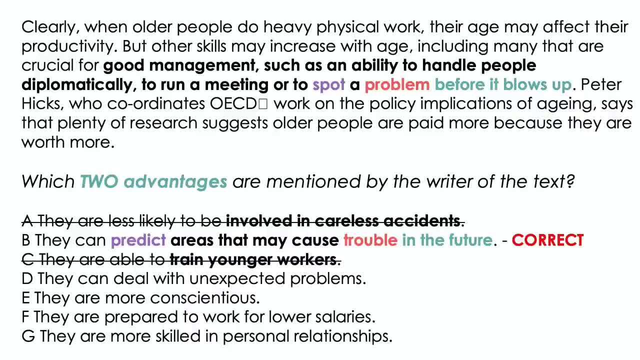 Nothing about it Incorrect. They can deal with unexpected problems. Ooh, look at this one. We've just read about problems in the paragraph. To spot a problem before it blows up, And we have an exact word match. The word problem doesn't mean it's a correct option. 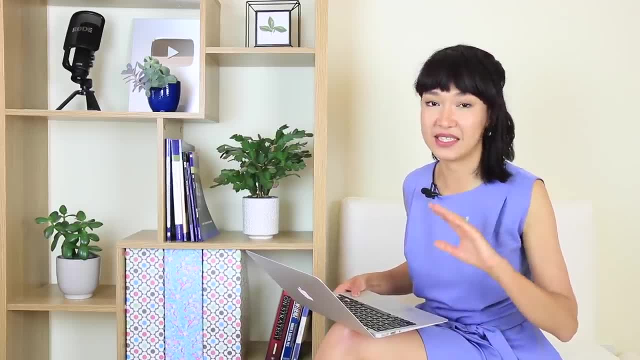 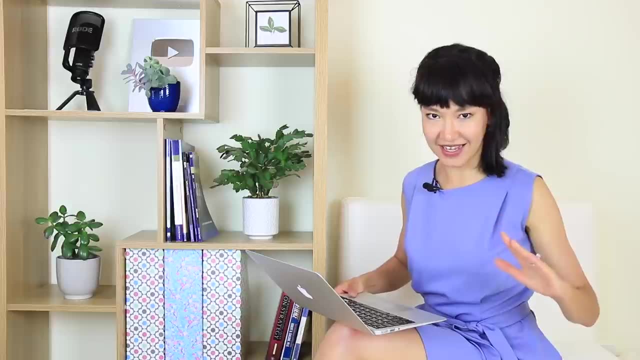 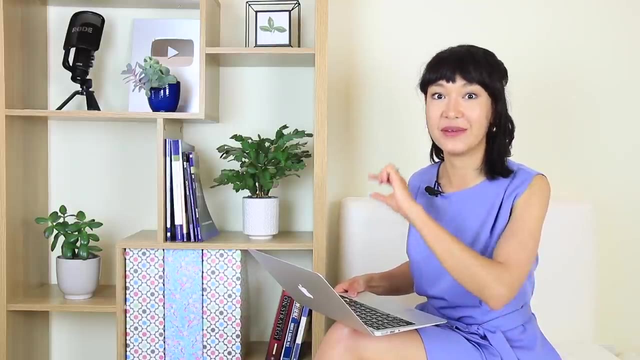 What I want to say is be very careful if you see the same words in the paragraph and in the options, In one of the options, Because most likely in IELTS correct answers are fully paraphrased. So all words are different but the meaning is the same. 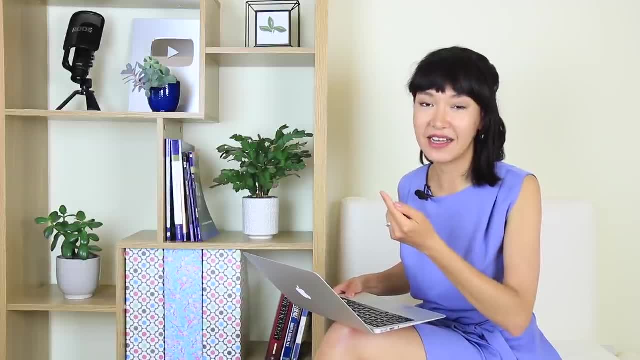 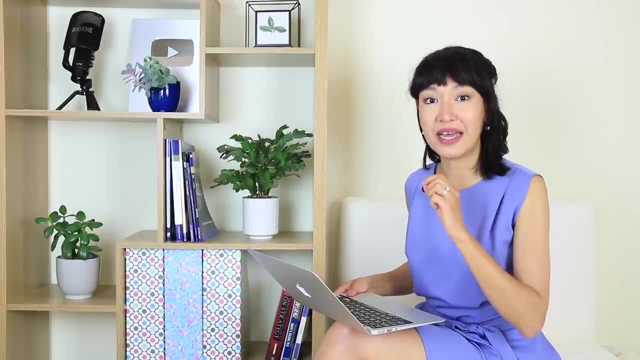 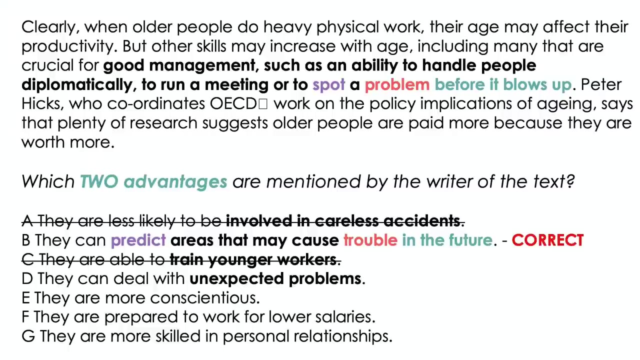 And options where words are repeated are usually just there to confuse you. It may be a trap, So you need to compare that the meaning of all the words in the statement is the same as in the text. Let's do that So we have deal with unexpected problems. 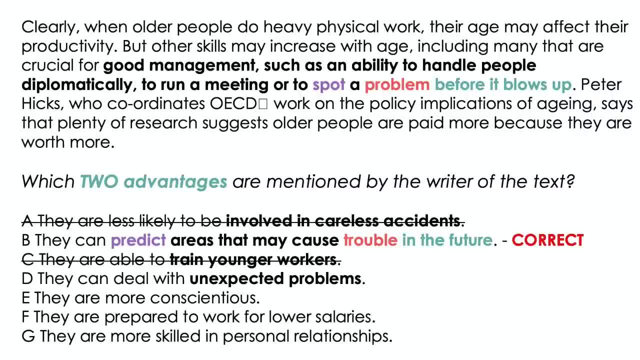 It means they can solve problems right, But in the paragraph we see to spot a problem, which means to notice, to discover a problem. So they don't mean the same thing. Let's look at the answer. B- Predict areas that may cause trouble in the future. 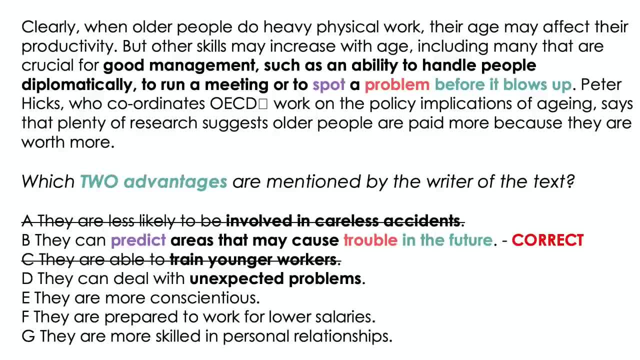 This means to spot a problem before it blows up. So in B, words are different but the meaning is the same- It's correct. And in D, the word problem is the same but the meaning is different And it's incorrect. As I mentioned before, 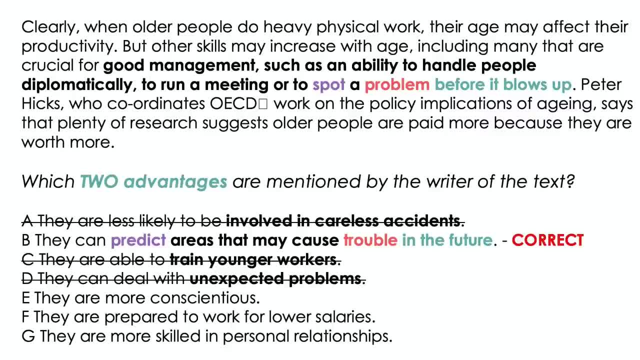 the correct answer is usually paraphrased and doesn't repeat the same words E They are more conscientious. Let's say we don't know what this word means. In IELTS reading you will find words you don't know and you need to know how to deal with that. 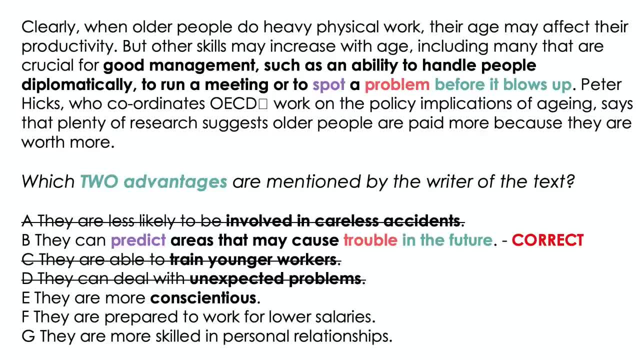 So in this case we can't say if the option is correct or not, And we just put a question mark and move on to the next option F: They are prepared to work for lower salaries. There is nothing about lower salaries, It's incorrect. 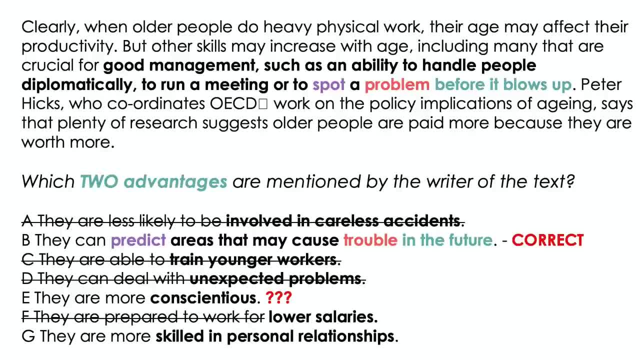 G, They are more skilled in personal relationships. Okay, and I can say that skilled in personal relationships means handle people diplomatically. So that's our second answer, And it doesn't matter that we don't know the word in option E. Try to concentrate on what you know. 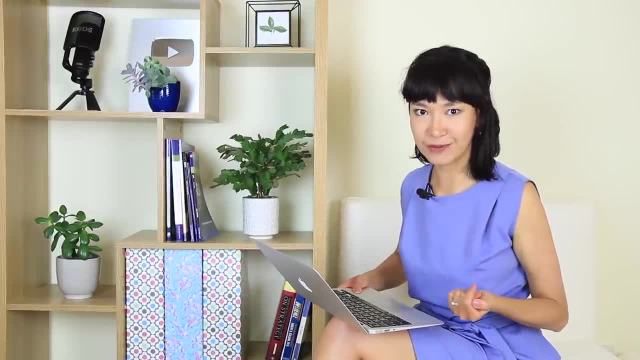 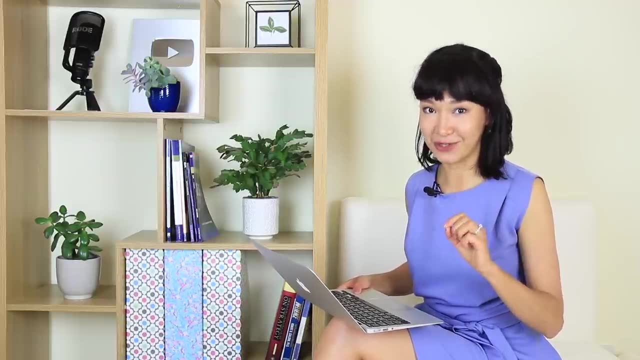 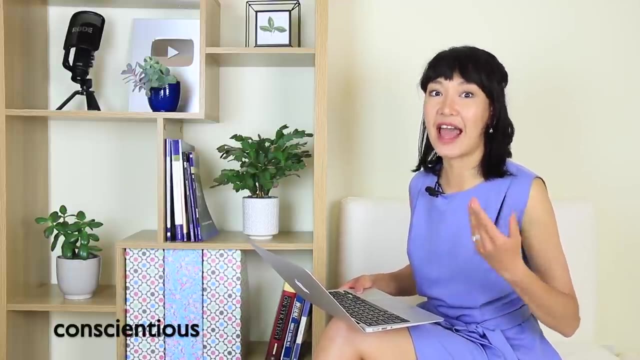 Try to check if other options are correct or not. There will be words you don't know in IELTS reading, but quite often you can still figure out correct answers. By the way, conscientious means taking care to do things diligently, accurately, carefully. 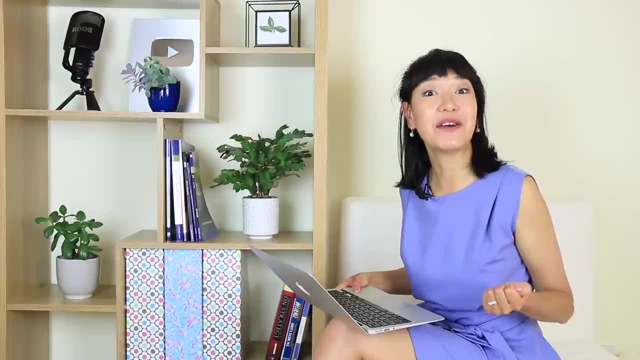 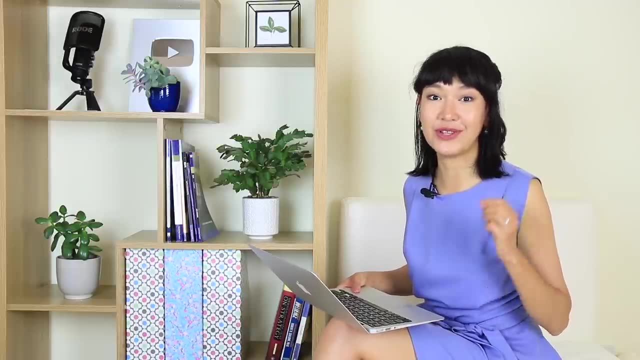 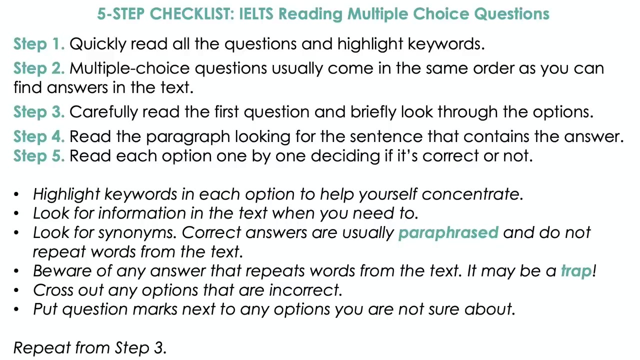 I've given you four questions so far. How many have you answered correctly? Please leave a comment. And now let's summarize the five steps you need to take to answer multiple choice questions. Step one: Quickly read all the questions and highlight keywords. 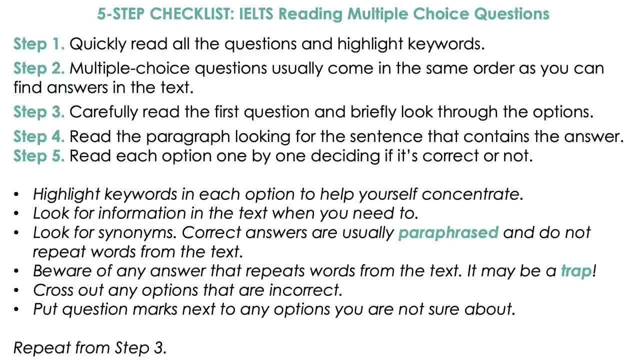 Step two: Multiple choice questions usually come in the same order as you can find answers in the text. Step three: Carefully read the first question and look through the options briefly. Step four: Read the paragraph looking for the answer to the question. 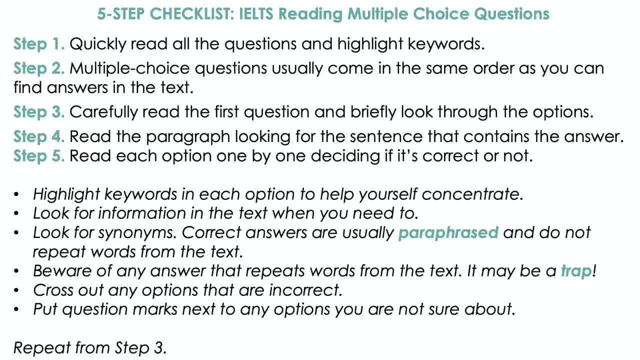 Don't worry if you can't see it. Just try to locate this sentence with the answer. Step five: Read each option, deciding if it's correct or not. Highlight keywords in each answer to help yourself concentrate. Look for information in the text when you need to. 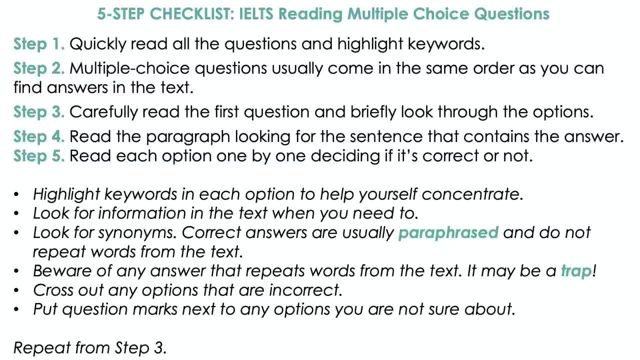 Look for synonyms. Words in the text and correct answers are usually paraphrased and words are not repeated. Beware of any answer that repeats the same words. It may be a trap. Cross out any options that are incorrect And put question marks next to any options you're not sure about. 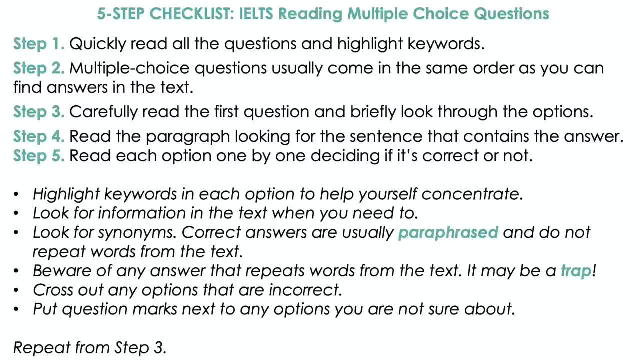 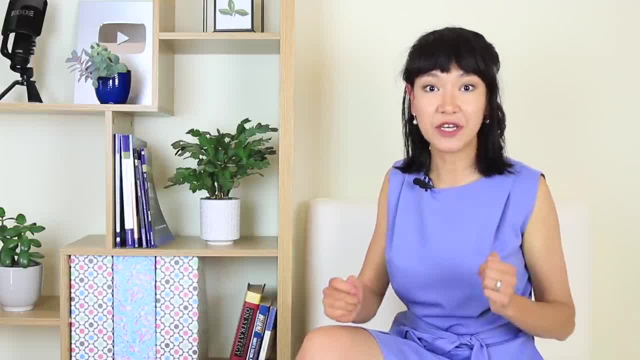 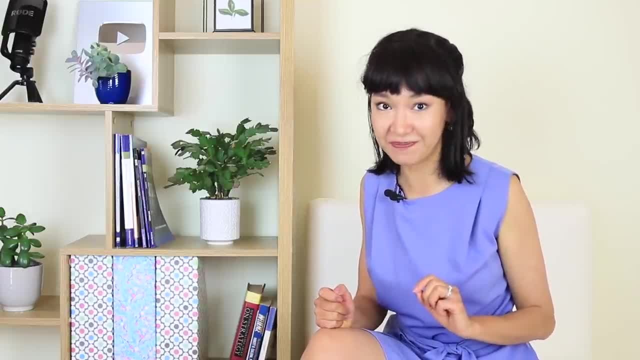 And for the next question, repeat from steps, Step three. These questions are taken from the official IELTS practice tasks and I'm going to link them in the description box below because you can find a couple of other questions I haven't shown you yet.